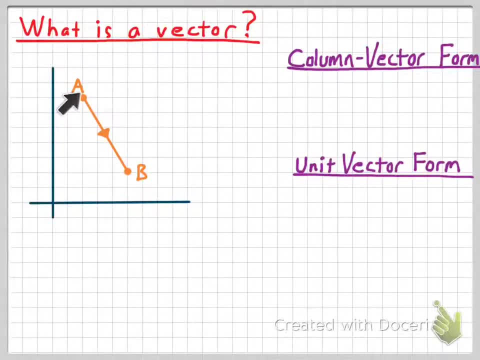 In that It is something that has a direction. I have a picture of a vector right here in two dimensions and you see this arrow right there indicates that this vector is traveling from point A to point B. Now it looks like a ray because you're traveling in a certain direction. 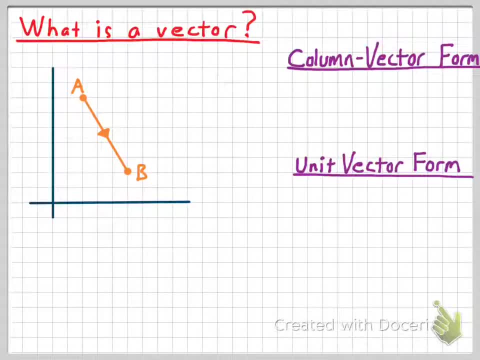 We're going from A to B versus from B to A, But a vector also has a certain distance, like a line segment does, So it's kind of a combination of a line segment and a ray. At any rate, the definition of a vector is that it's a quantity that has size. 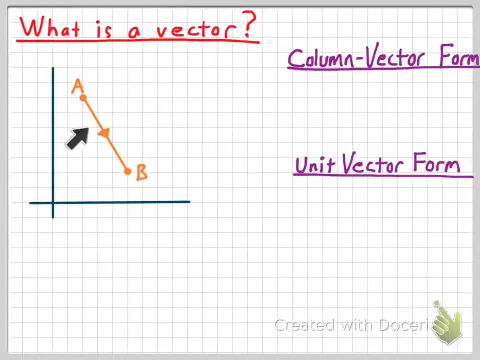 And Direction, And here you have something that has a size because it has a length and it has a direction because it's going this way. Now, the direction of the vector is what we use to represent the vector in one of two different forms: either column vector form or unit vector form. 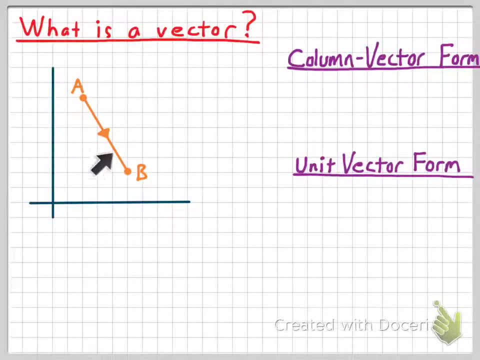 And so let me describe how that works for you. First of all, notice if we're going from A to B. you could describe the direction that it's going by telling how far horizontally you go, what the horizontal change is from A to B, and then what the vertical change is from A to B. 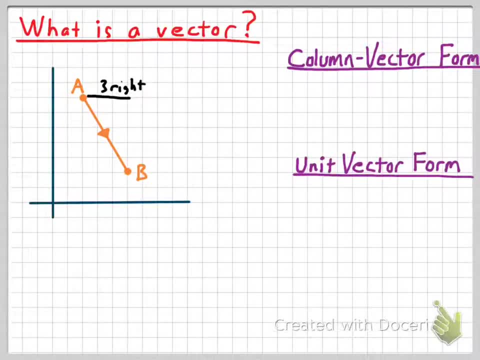 And in this case that would mean that you go three units to the right and four units down. And, very simply, whenever we're trying to represent a vector, we want to say what's the horizontal distance and the vertical distance you travel to get from the initial point to the terminal point? 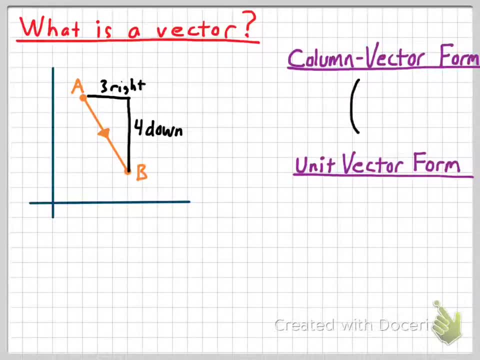 And if you want to represent that in column vector form, all you do is you make a set of parentheses and you put the horizontal component first. We went three to the right, So this is positive. Had we gone left, that would be negative. 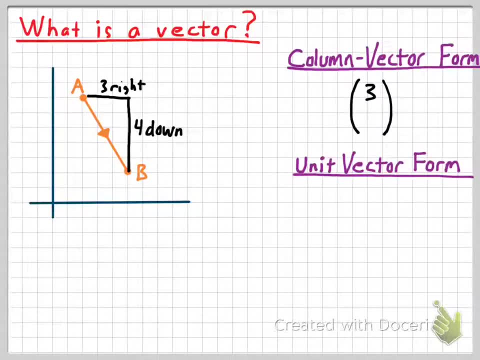 And then you put the vertical component right underneath that. We went down, So we're going to call that negative four. Had we gone up, it would have been positive four. All right, Then for the unit vector form. I need to add some information to your screen real quick. 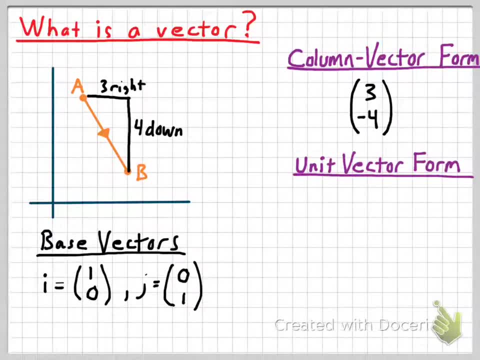 You say. I wrote something about what are called base vectors down here and I'll come back to that. A unit vector is simply a vector that is one unit long, just like a unit circle has a radius of one. All right, A unit vector is one unit long. 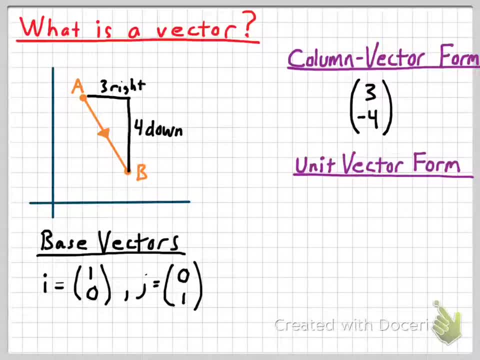 Because, remember, vectors have size and direction. That's the size. Now there are two special base vectors, what are called base vectors, that we use in two dimensions, which is what we're working with. right, there is two dimensions that we use. 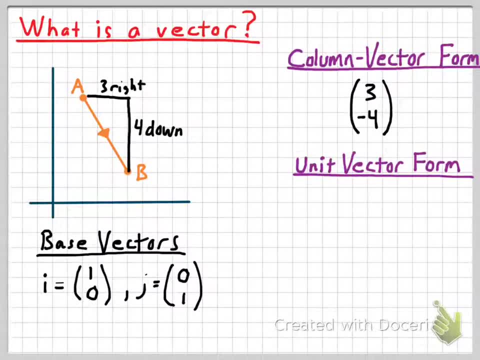 We have one called I, which is one comma zero And so base vector. I would look like this if you graphed it. Don't know how well you can see the direction there, but that's one unit long and it's going to the right. 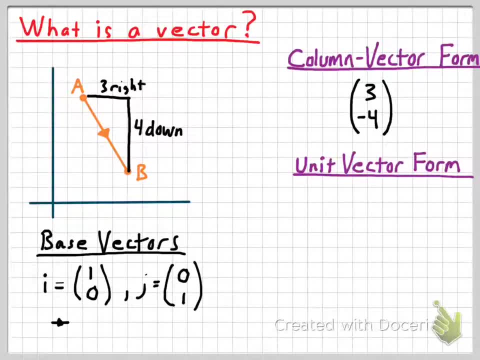 Doesn't go up or down at all, And there's a base vector, J, that goes zero units horizontally but one unit up. so it would look like this And what we can do is we can take any vector and we can represent it using these base vectors. 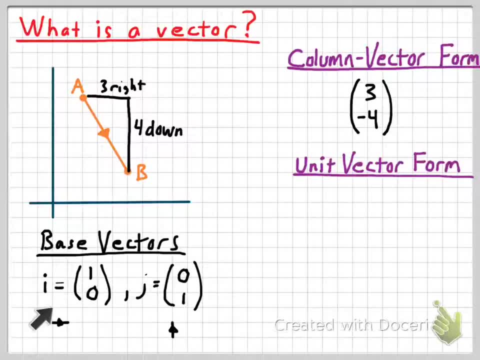 by simply saying that you're going three of these minus four of those. right, We went right three times, so we went I three times, and then we went down four times, so we went J negative J four times. We can write then this vector: 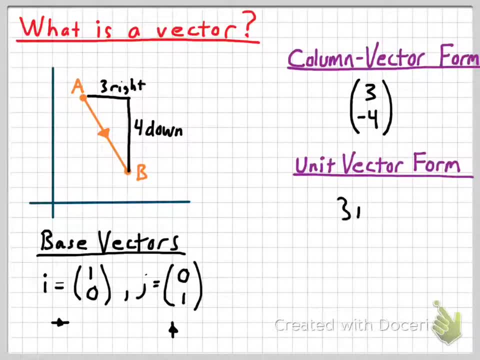 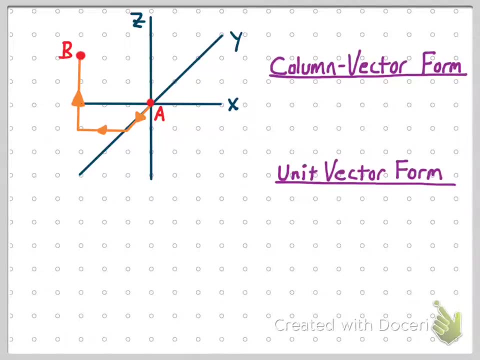 As three I minus four J. All right now, that's two-dimensional vectors. I want to give you an idea of what three-dimensional vectors are and how to represent them using each of these forms as well, And we have to use what's called a coordinate space in order to make a picture of those. 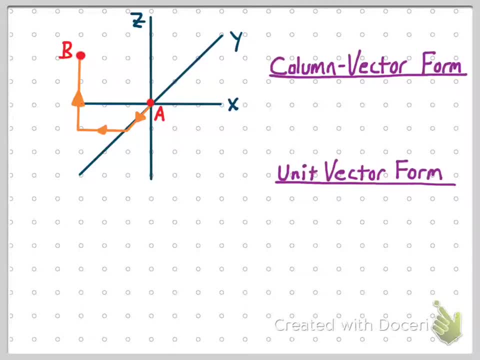 Now I've drawn such a coordinate space here. You can see it's got an X and a Y and a Z axis and I'm going to label something really quickly. All right, you see the X axis is positive, going to the right. 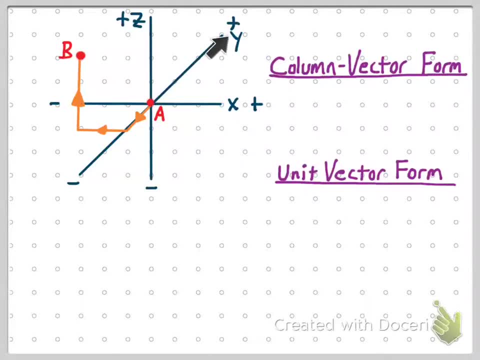 And negative going to the left. The Y axis is positive as you go back And it's negative as you go towards yourself, so to speak, And the Z axis is positive going up and negative going down. All right, now I'm going to try to represent a vector AB here. 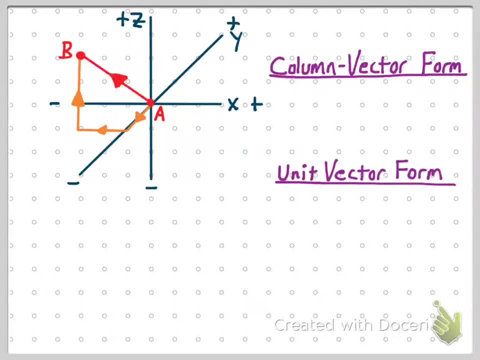 That would go from there to there, And in order to write down its column, vector or unit form, we need to break down its components, And it has three components, because it was well in three dimensions, right. So first of all, we can say that this thing went either left or right. 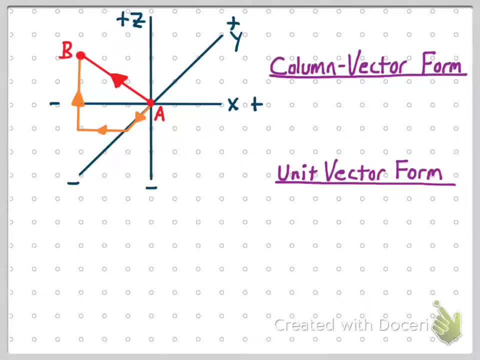 We can say it either went towards you or away from you, And we can either say it went up or down, And in the column vector form we care about the left or right or the X coordinate first And you can see that this thing goes one, two units to the left.